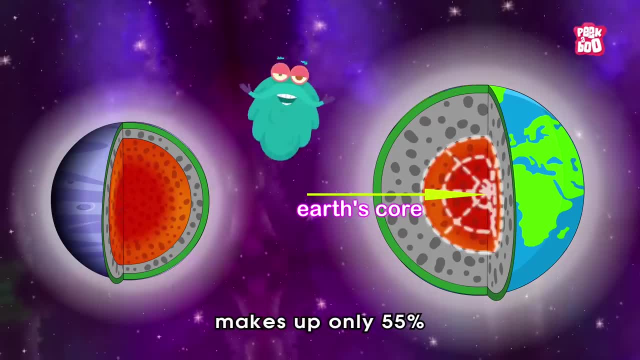 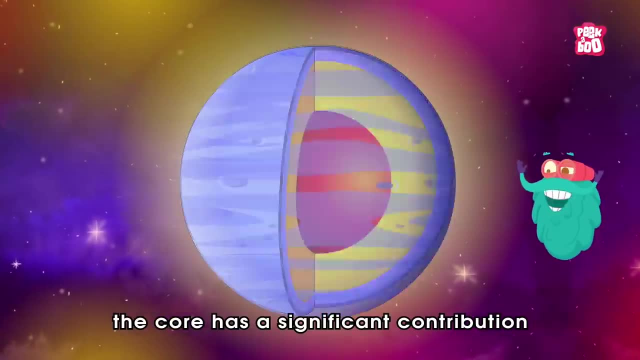 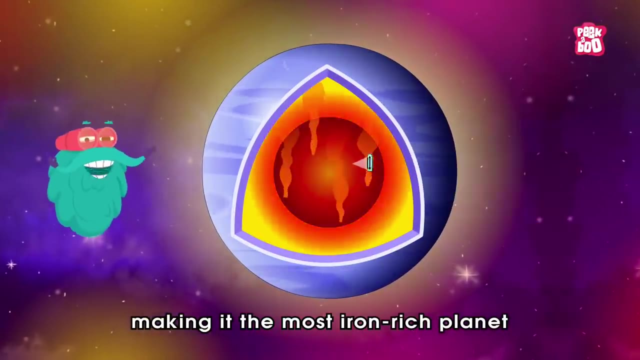 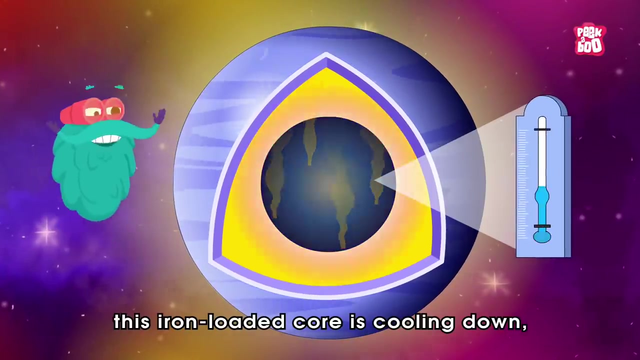 While the Earth's core makes up only 55% of its total size. Also, the core has a significant contribution towards the weight of Mercury, Making it the most iron-rich planet in the entire solar system. But with time, this iron-loaded core is cooling down, resulting in the wrinkling and shrinking of this planet. 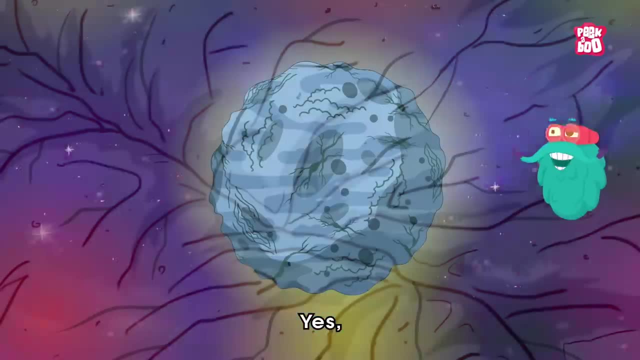 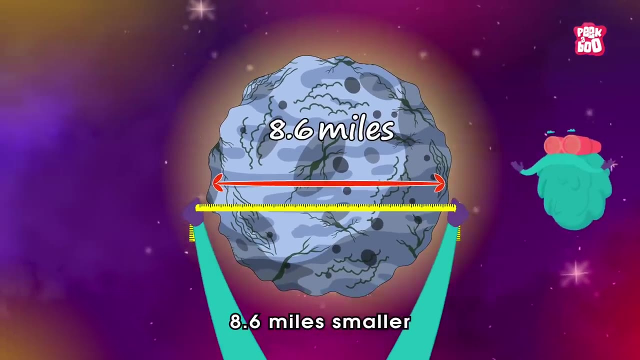 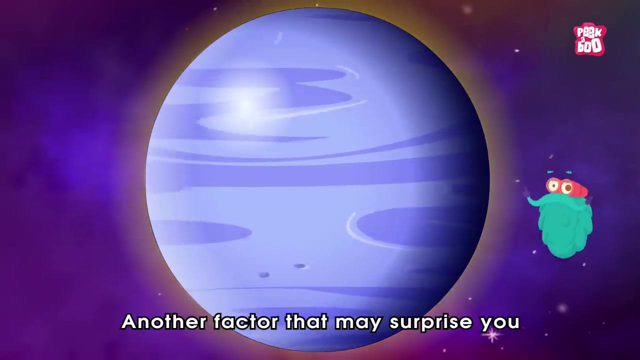 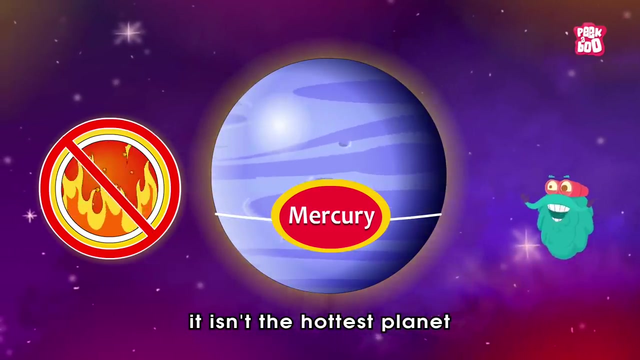 Like a raisin. Yes, some scientists estimate that the planet is now about 8.6 miles smaller in diameter than it was nearly 4 billion years ago. Another factor that may surprise you about Mercury is that it isn't the hottest planet in our solar system, despite being closest to the sun. 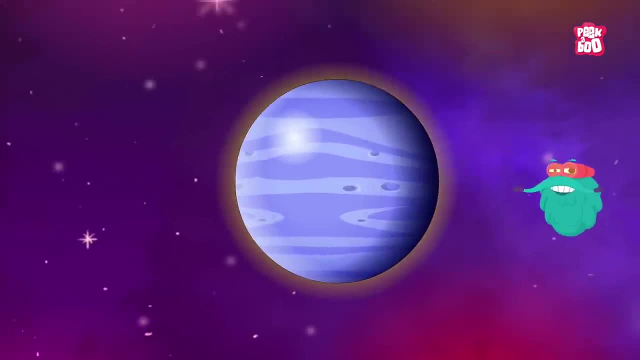 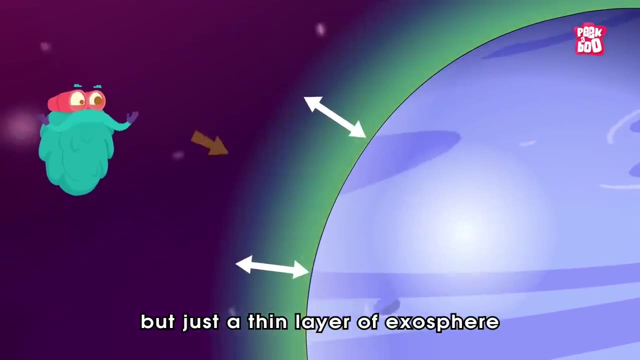 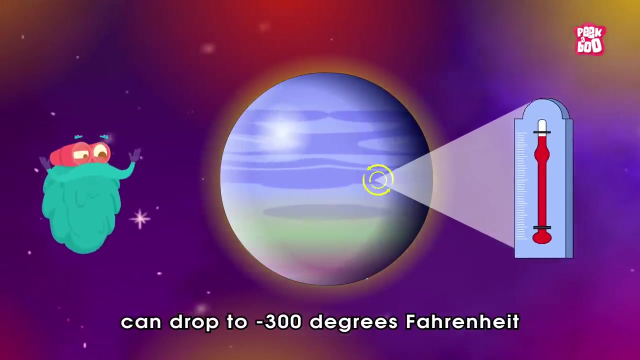 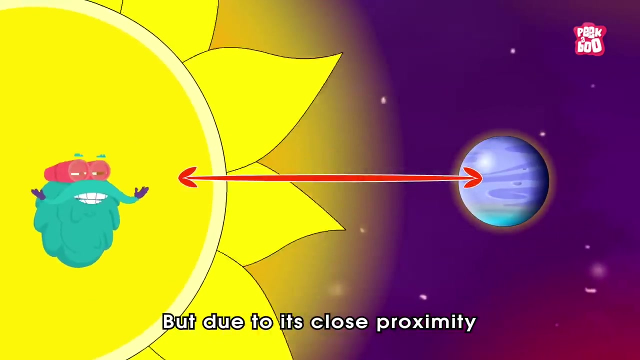 Yes, because it has almost no atmosphere, but just a thin layer of exosphere that cannot hold in heat and keep the surface warm. The temperature can drop to minus 300 degrees Fahrenheit during nights, But due to its close proximity to the sun, it can rise up to a whopping 800 degrees Fahrenheit. 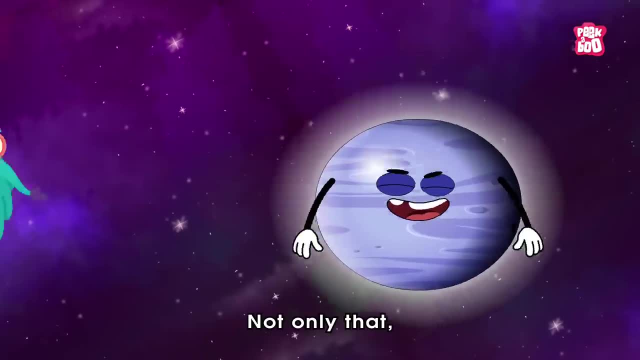 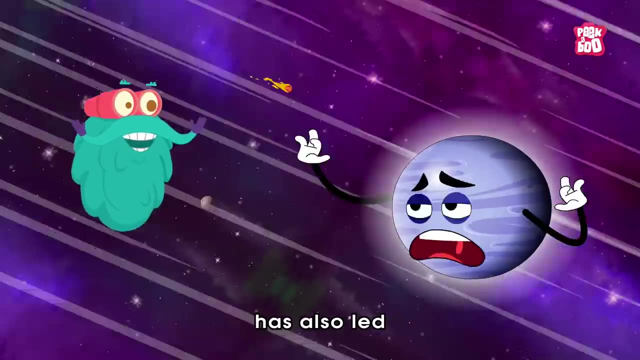 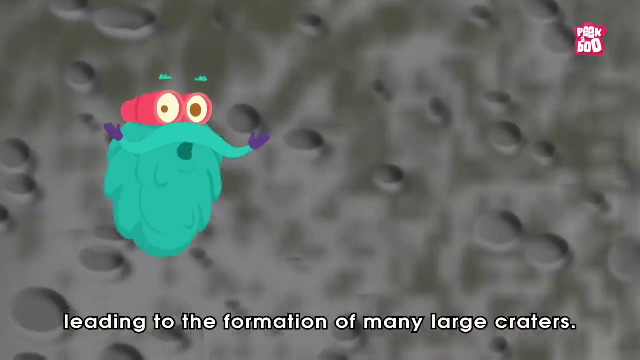 During the daytime. Not only that, but this lack of an atmospheric layer to protect it from the outer attacks has also led to multiple meteor showers on this planet, Leading to the formation of many large craters, One of which is called the Calaris Basin. 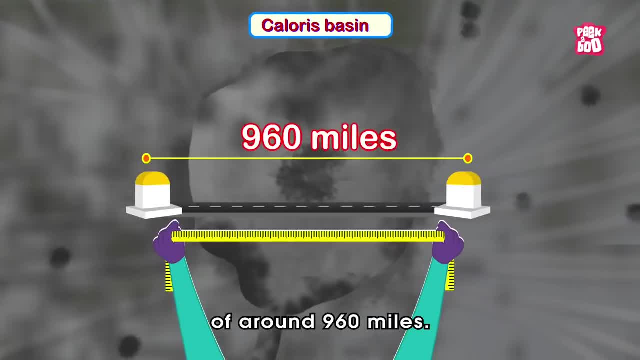 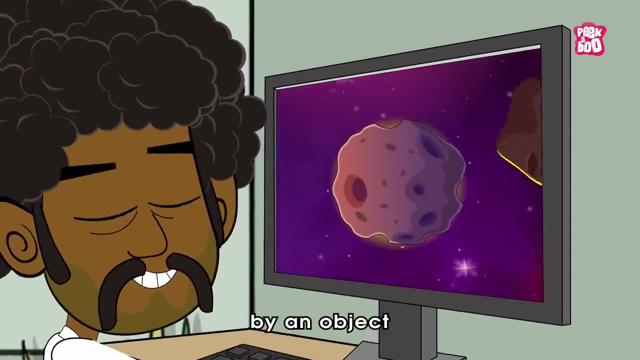 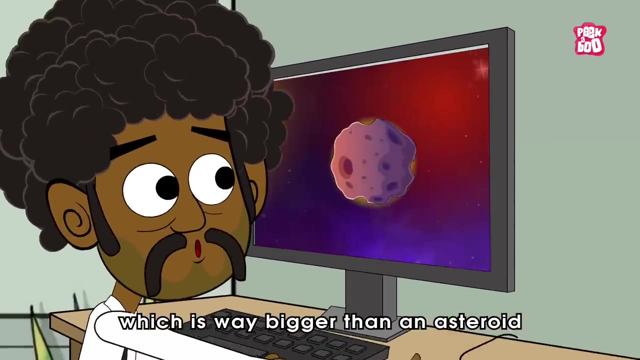 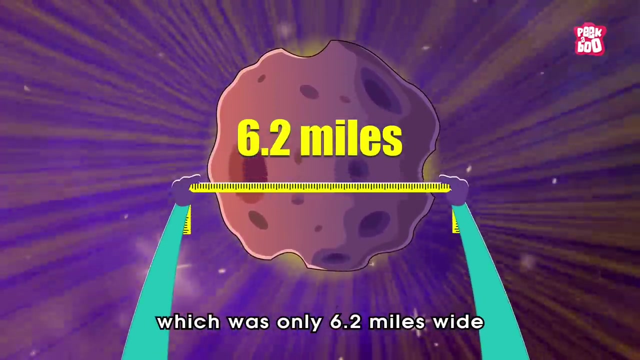 Which has a diameter of around 960 miles. Researchers believe it could have been caused by an object nearly 62 miles wide, Which is way bigger than an asteroid, ChickX Club impactor, Which was only 6.2 miles wide but still managed to wipe out dinosaurs on earth.